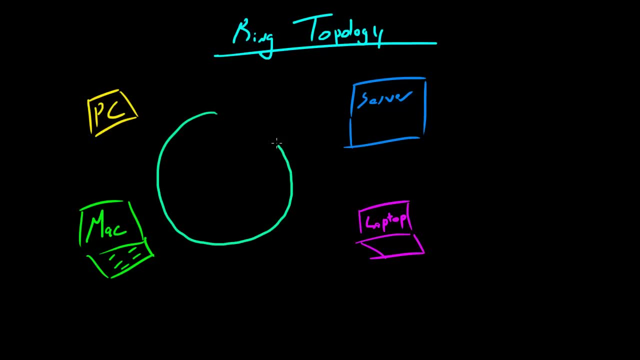 well you can remember, because on these devices are connected to one main ring. so say that this is ethernet and this is your main ring, and this is of course all ethernet cord right here. and obviously, if you were to put it in your house it wouldn't be in the shape of a perfect circle, but the entire. 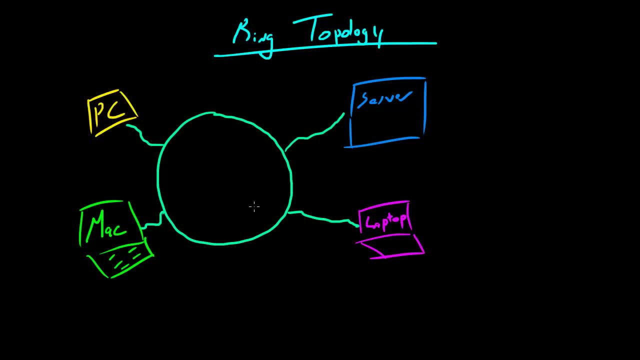 layout. if you step back and look at the you know diagram, it will look like it's all connected. all your devices are connected to a basic ring system. so, first of all, we notice that there are no terminators. why is that? well, it doesn't have a logical beginning in the end of a ring, just like a circle. so you don't. 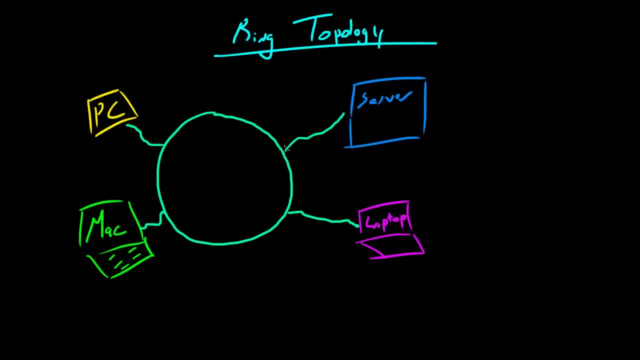 need anywhere to terminate it. so that's why it's beneficial or better than a bus topology. another thing is that, well, if we look at how data is logically, logically transmitted, say that this laptop or say that this Mac right here wants to access this server over here, so what it would do is it would send out a request, basically. 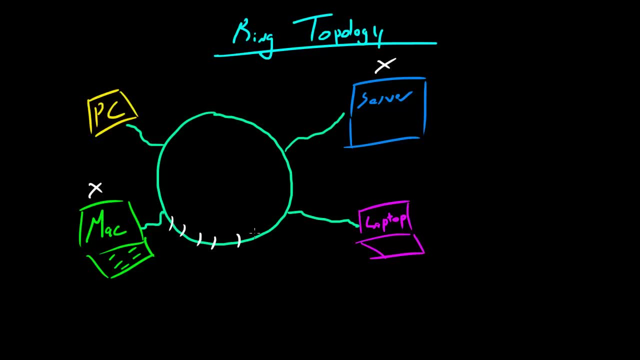 send out data and this data would go around the ring in one direction. in it hit each node at a time. so at first say, okay, laptop, do you have the file that I'm looking for in the laptop? is gonna be like dude, I'm not a server, so he's. 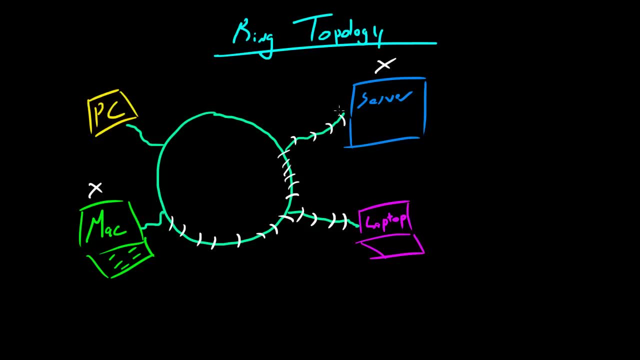 going like: okay, okay, here we go the server right here. server, do you have the information that I want? and the servers gonna make, yeah, buddy, I do. and then it's gonna keep going because you know, this is an electrical signal and it goes everywhere. so it's even gonna ask the PC, even though it already got the 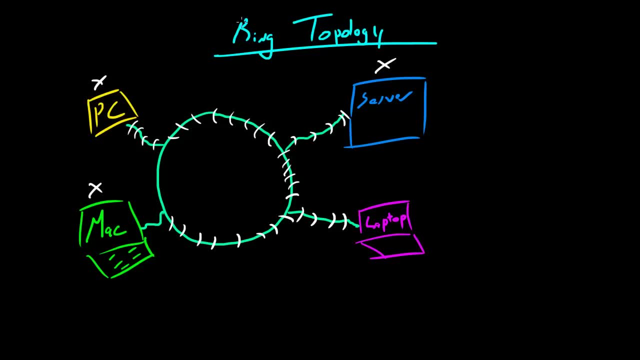 information from the server. that's you know part of the thing that you need to understand about a ring topology. it hits node by node and even if it reached the destination that it wanted to reach, it continues along until it returns to the source node. now again, as you can see, it doesn't really reach an end. 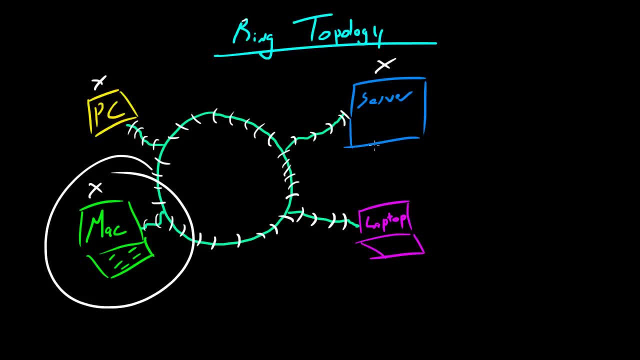 point. it just flows in one main direction and eventually it gets what it wants and it always comes back to the source node. so that's, overall, how this ring topology works. now, even though this is typically the way it works, the way they are actually built is there are. let me just go ahead and draw this real quick. 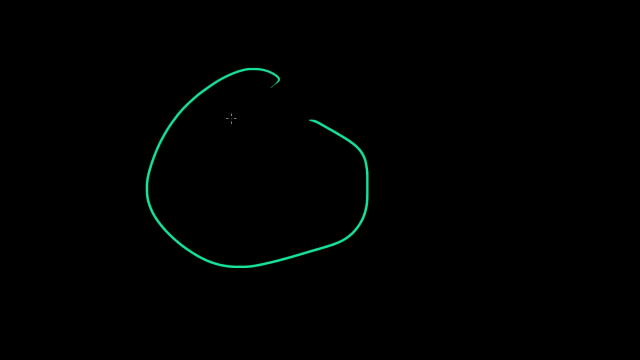 you actually have two rings: one- yeah, I can try that a little better- one right here and another one basically right beside it, and whenever we have this, say we have four devices- one here, one here, one here and one here. the way that these are typically built is: you can go ahead and 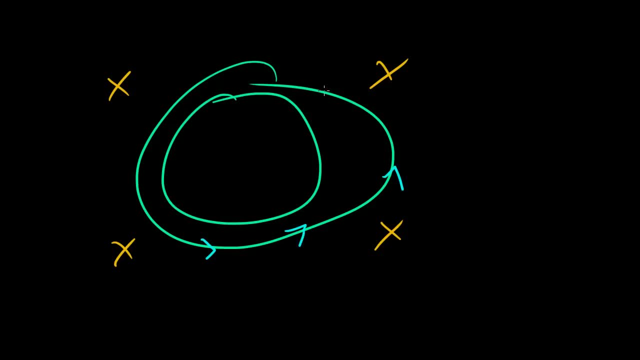 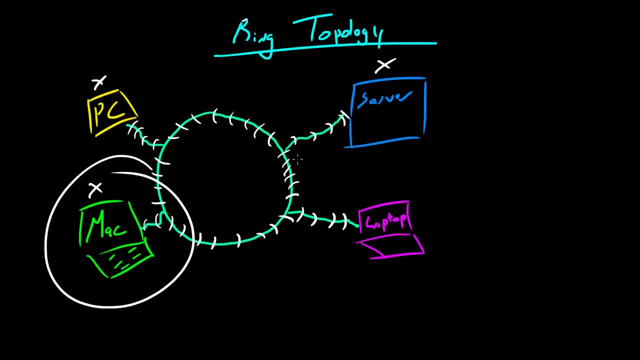 set up two rings where the data flows in this direction on one of the rings and in the opposite direction on another ring. so we call both of these, you know, topologies, ring topologies, even though this one is, you know, a very simplistic ring network. and this one right here is a more common one, where they have two rings and the. 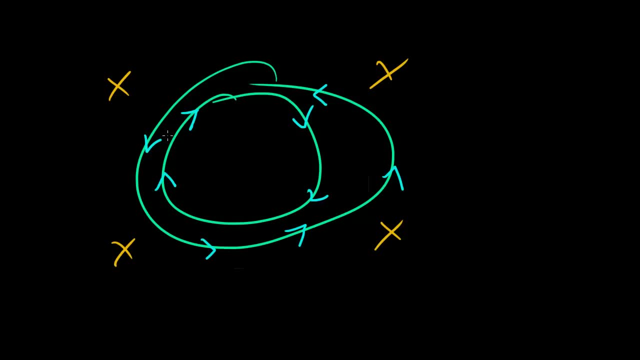 data can flow in opposite direction. and it's also better because if the ring breaks in, this network will say we'll call this the double ring network. if one of these rings breaks or the Ethernet breaks on it, then your network is still going to work. so that is, this is actually in fact called the ring. 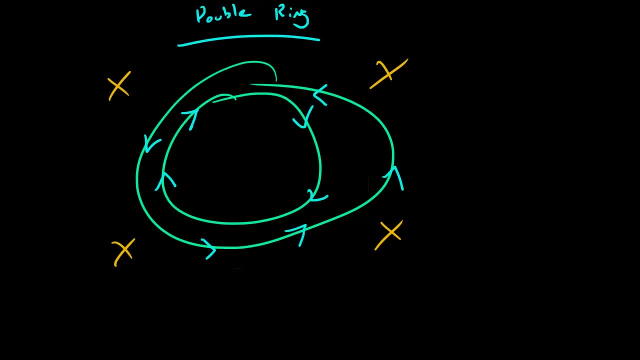 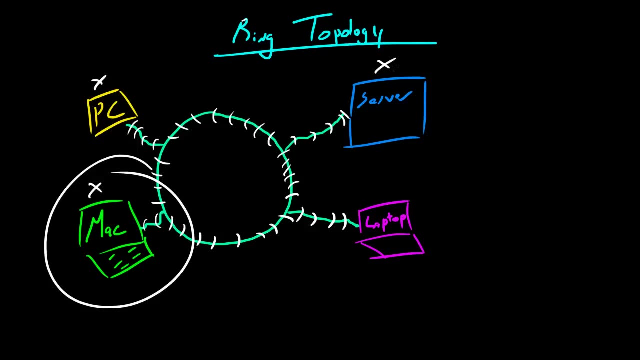 topology as well, but I'm just going to call it a double ring to differentiate it from my single ring. but basically, overall in the ring topology it's better than a bus topology because it can hire, handle volumes of data better than a bus. but the negative part about it is it's usually- let me get a good color here. 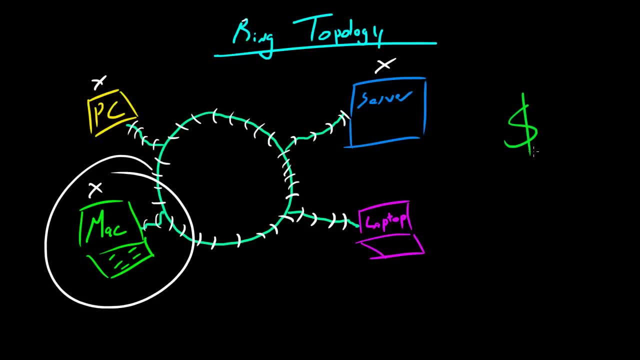 it's usually a lot more expensive than a bus topology. so if you're choosing between, you know, a bus and a ring for your home network, if you're not worried about money, then I would go ahead and go with a ring topology or you could go with a bus topology. but if you are worried about money, then you can go with. 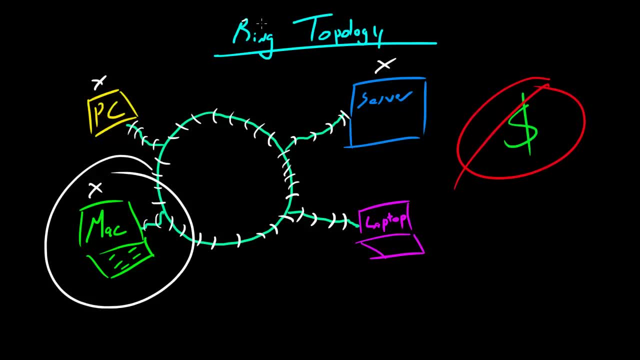 a bus topology. but if you have a lot of volume, then I would definitely recommend getting a ring until you see my next videos, because in my next couple videos I'm gonna be showing you guys the most common type of topology and this is probably the one that you have in your home right now. but for now- now we know- 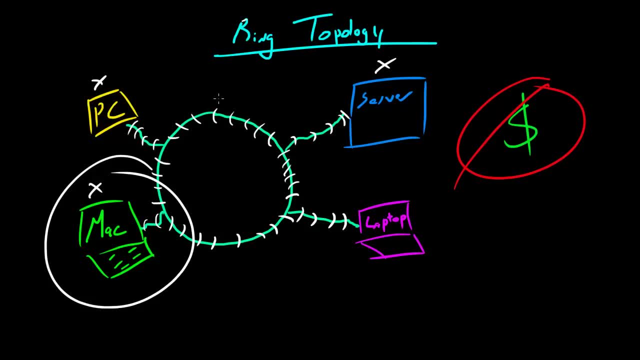 between you know the differences between a ring and also a bus. basically, a bus, very simplistic, has terminators. a ring is usually built with two rings so data can flow in either direction. handers higher, higher volumes, better, but is usually more expensive. and, by the way, don't forget to.